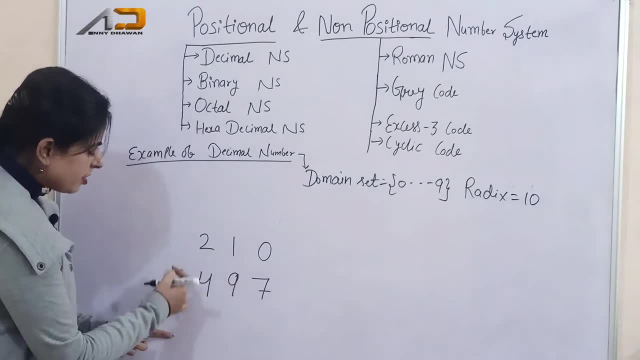 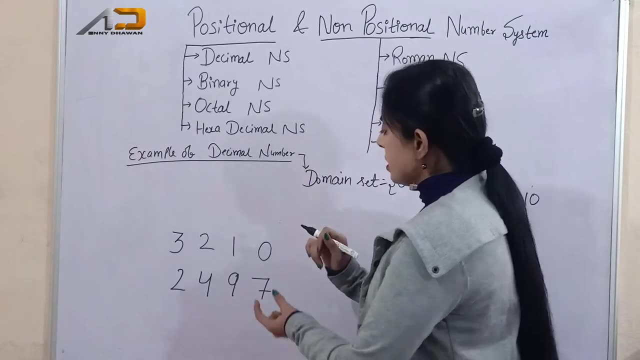 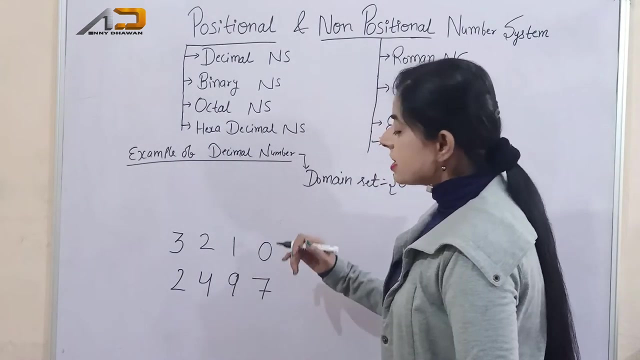 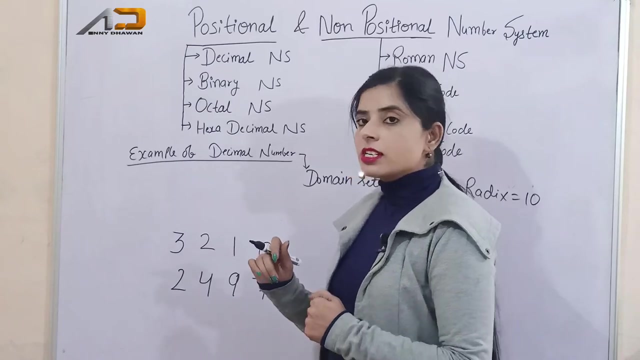 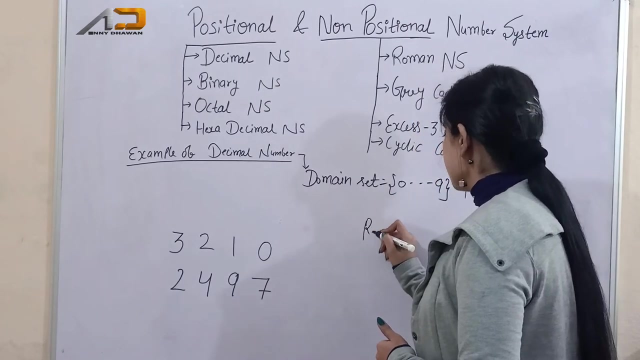 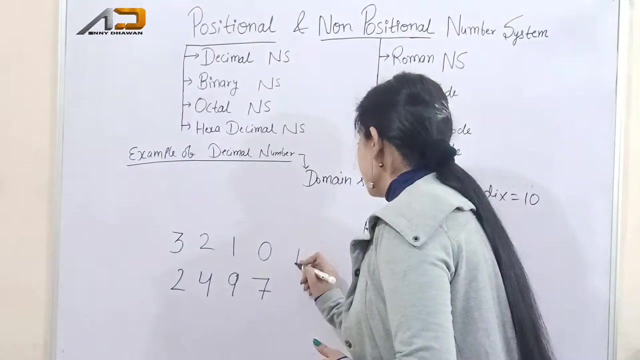 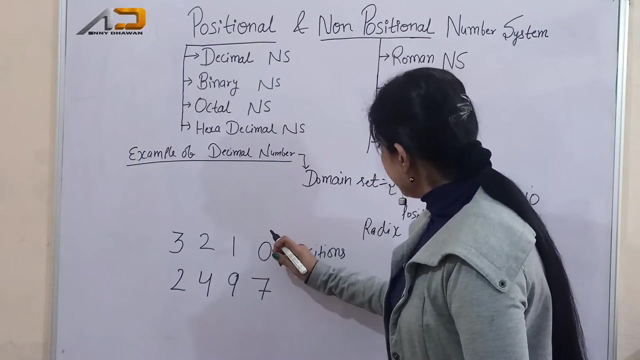 What is the position of 4? here is 2 and the position of 2 is 3, and in positional number system, this specific position in turn has its corresponding significant, or you can say weight value. And now the question is: how can we find the weight value and the formula for finding the weight value: is red X raised to the power position? What are the positions here? These are the positions and how can you find the corresponding weight value. is red X raised to the power position? 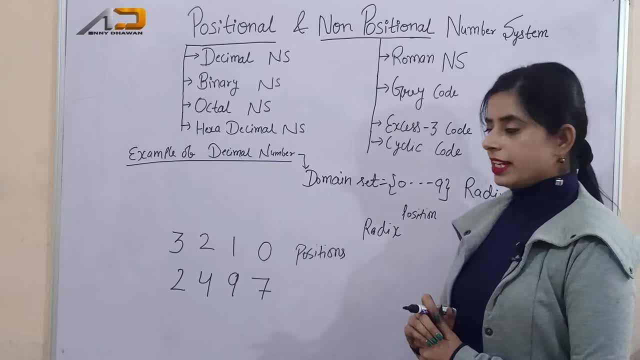 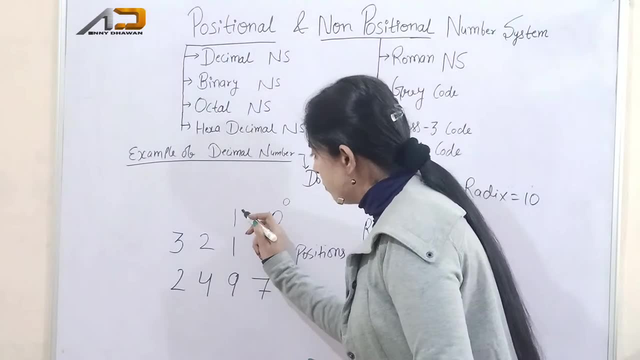 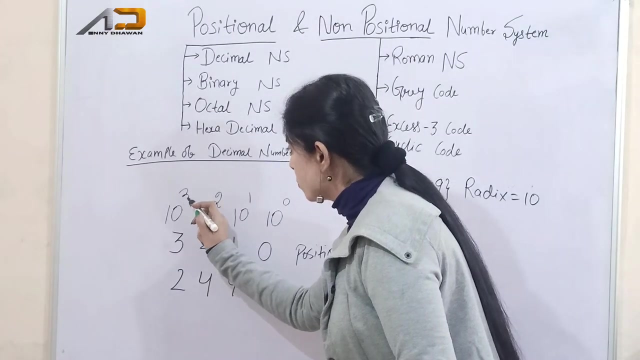 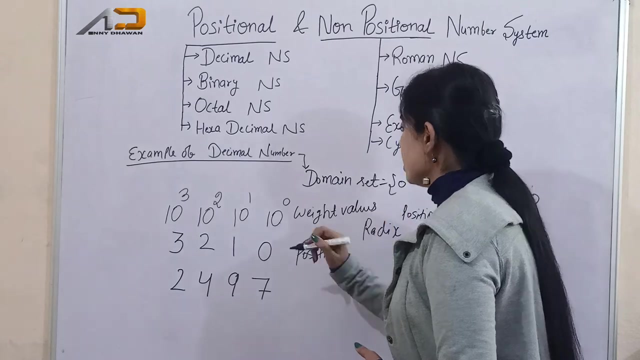 What is the weight value? So the red X of decimal number system is 10.. So the weight value would be 10 raised to the power 0, and next weight value would be 10 raised to the power 1.. Next weight value would be 10 raised to the power 2, and next weight value would be 10 raised to the power 3.. So these are the weight values, or you can say significant values. 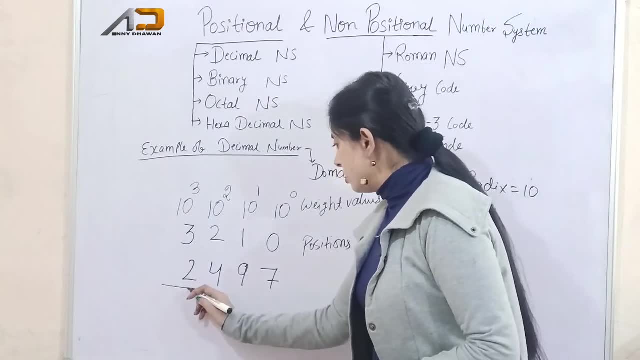 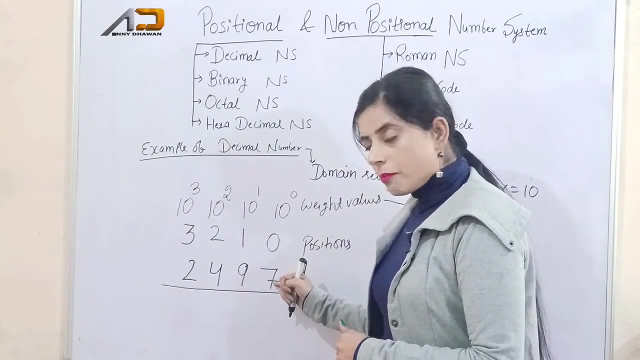 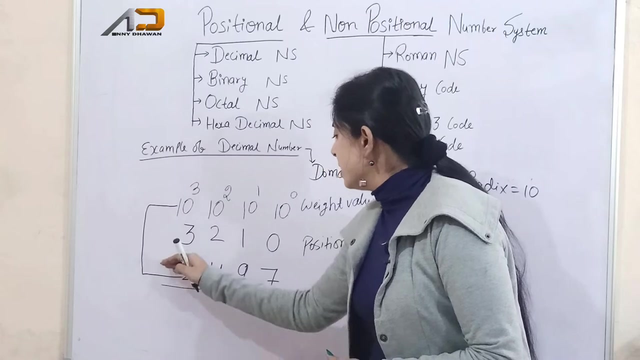 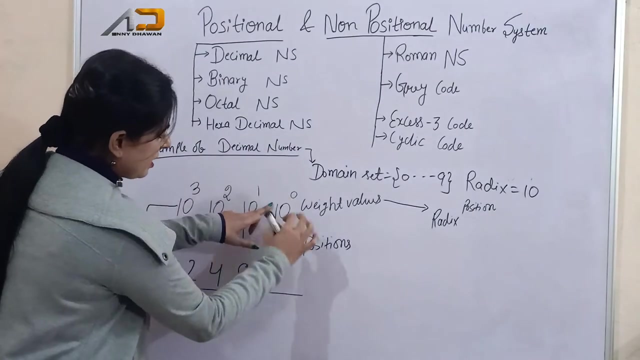 Now find the value of each of the Position. and how can you find the value of each of the position? multiply the digit itself by its corresponding weight value. that is, You have to multiply these digits by their corresponding weight values. that is, 7 multiplied by 10 raised to the power 0, you will get 7. 9 multiplied by 10 raised to the power 1, you will get 9.. 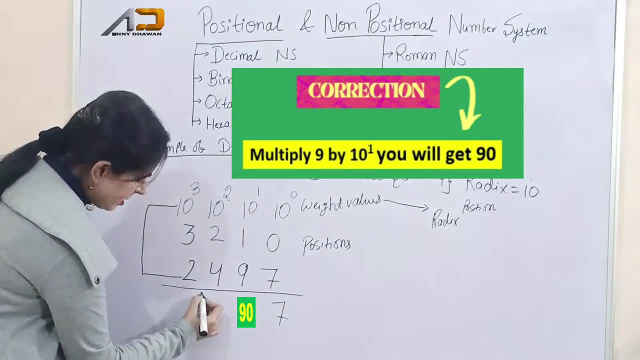 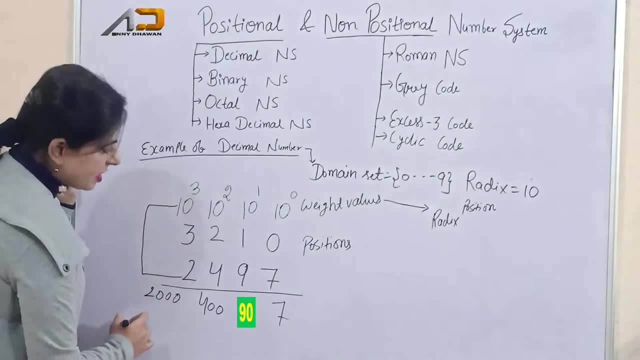 4 multiplied by 10 raised to the power 1, you will get 9.. You will get 9. and to 10 raised to the power 2, you will get 400. and 2 multiplied by 10 raised to the power 3, you will get 2000. and to get the final answer, add the values of all the positions. 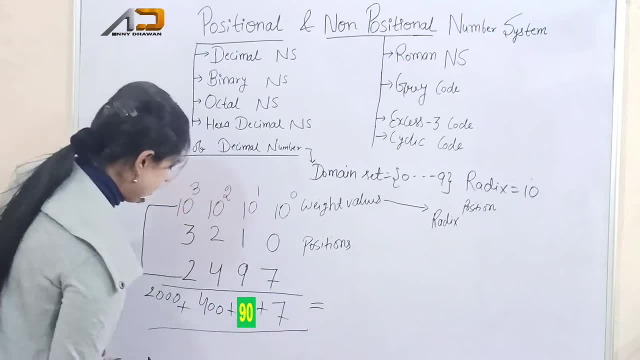 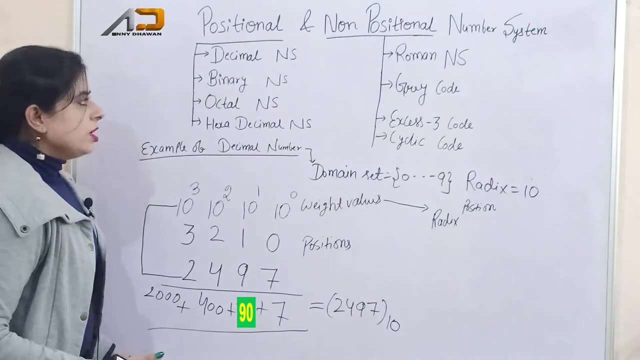 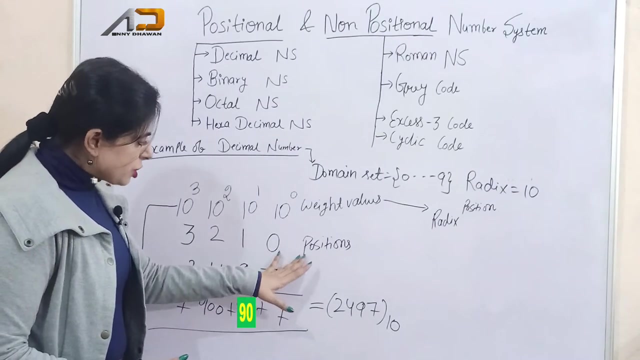 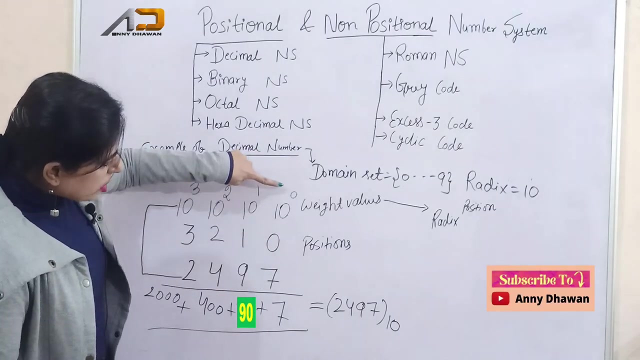 And you will get the number 2, 4, 9, 7 to the base 10.. So in positional number system every digit digit ki ek specific position hoti hai, Aur uss position ke corresponding digit ki ek corresponding weight value hoti hai, Aur wo corresponding weight value hum kaise find? 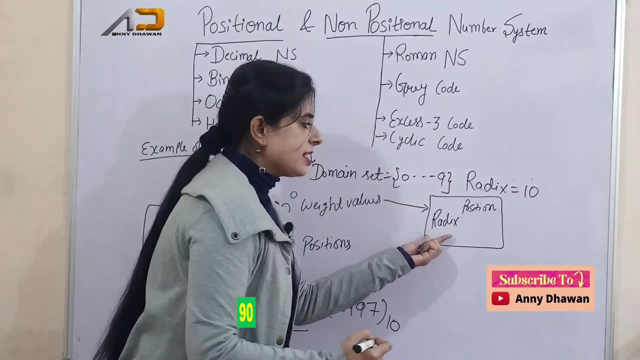 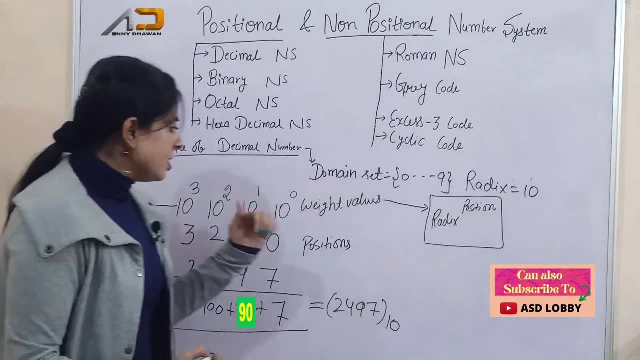 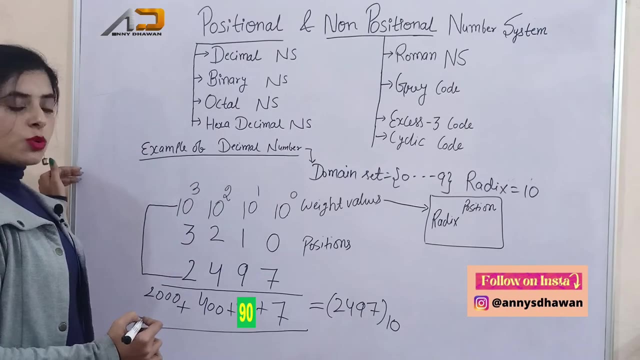 kar sakte hai Uska formula? kya hai Radix raised to the power position? Aur yahan decimal number system me radix kitna tha 10.. So weight values kaise niklengi humari? 10 raised to the power 0,, 10 raised to the power 1,, 2,, 3 and so on. Now I am going to take one. 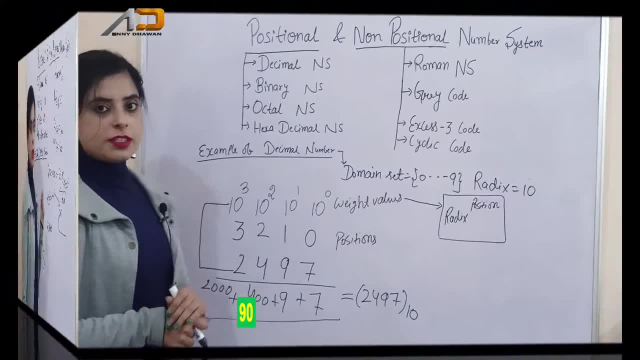 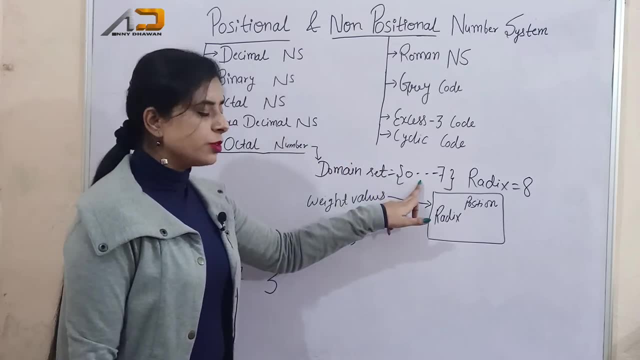 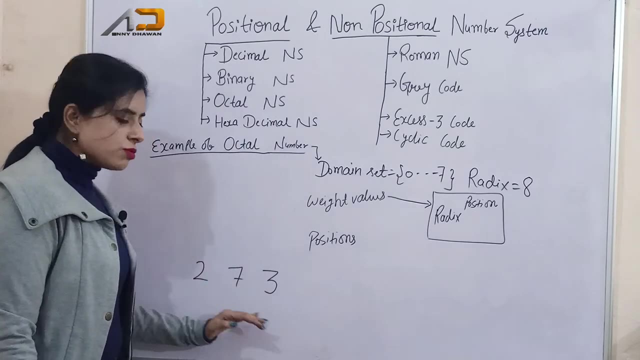 more example of octal number system. All of you already know that the domain set of octal number system includes 0 to 7 digits and radix of the octal number system is 8.. I have written a number here that is 273 and it's a valid octal number as all the 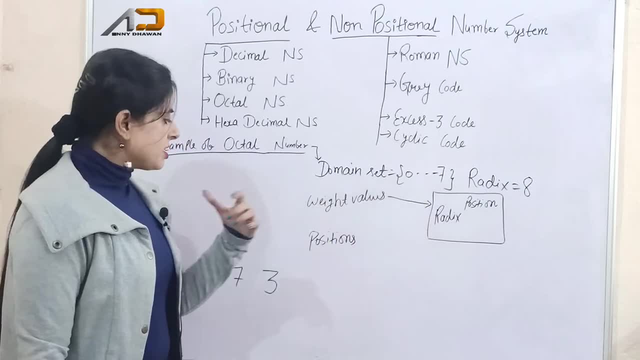 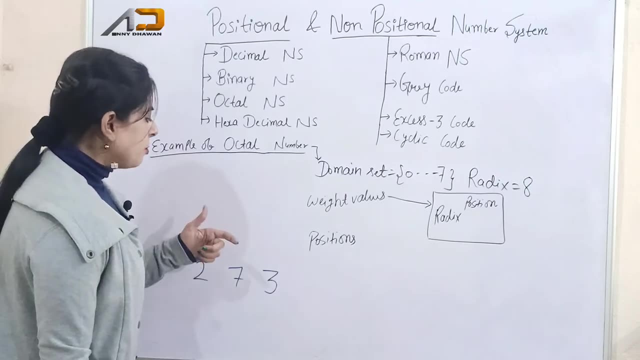 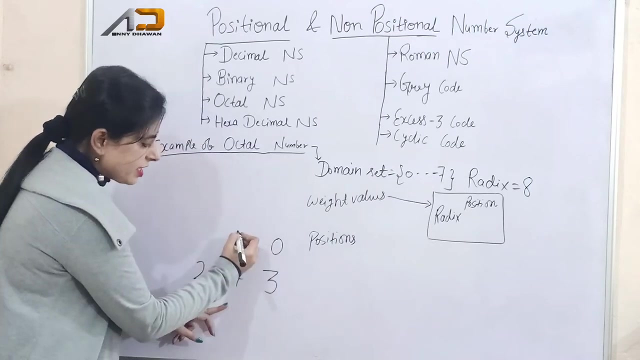 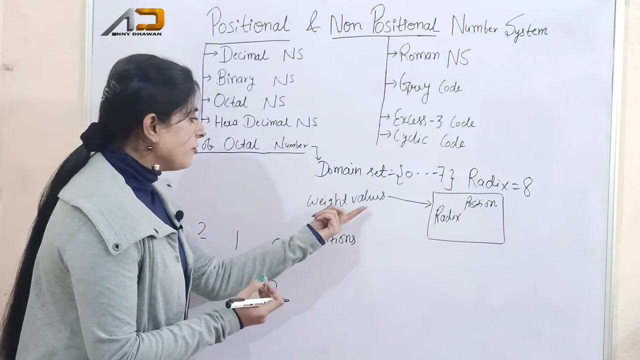 digits belong to the domain set of octal number system And now follow the same process that I just explained, That is, write the position of each of the digit, That is, the position of 3 is 0,, the position of 7 is 1 and the position of 2 is 2.. Now find the corresponding. 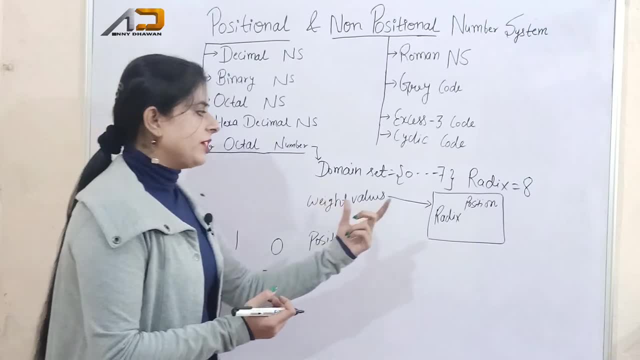 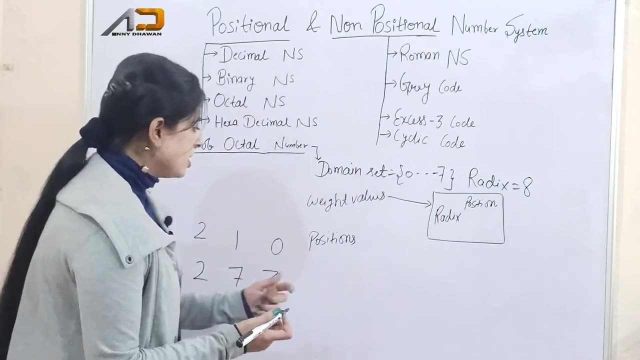 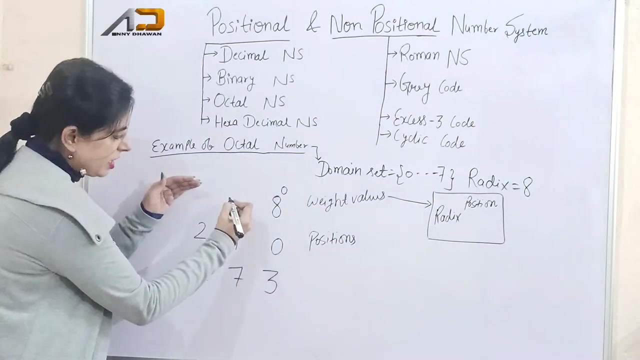 weight value of each of the position. You can find the weight value by using this formula. that is: radix raised to the power position. What is the radix here? 8.. Now the weight value would be 8 raised to the power 0.. For this position, the weight value would be 8 raised. 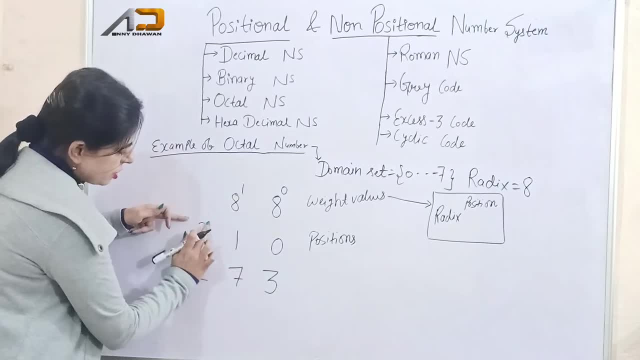 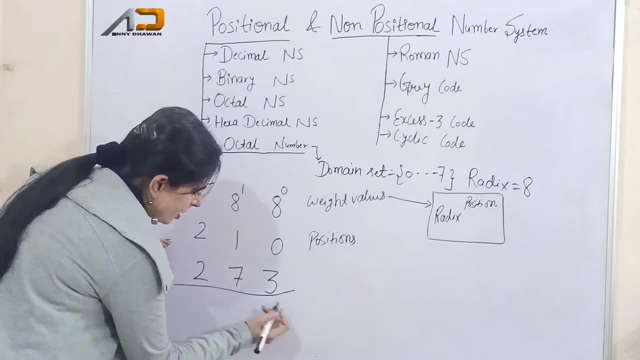 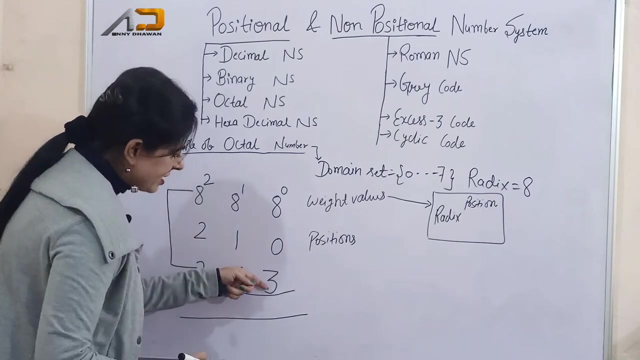 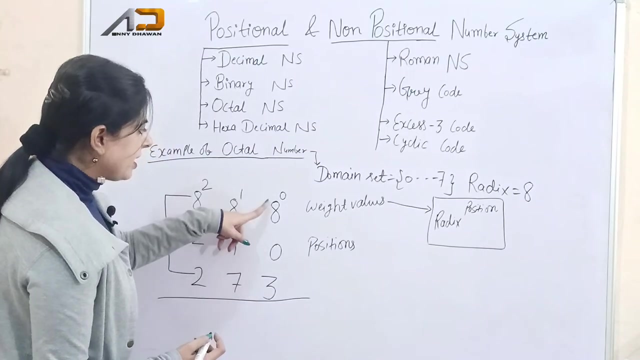 to the power 1, and for this position the weight value would be 8 raised to the power 2.. And how can you find the value of each of the place? Multiply the digit itself by its corresponding weight value, That is, multiply 3 by its weight value, 8 raised to the power 0, and you will. 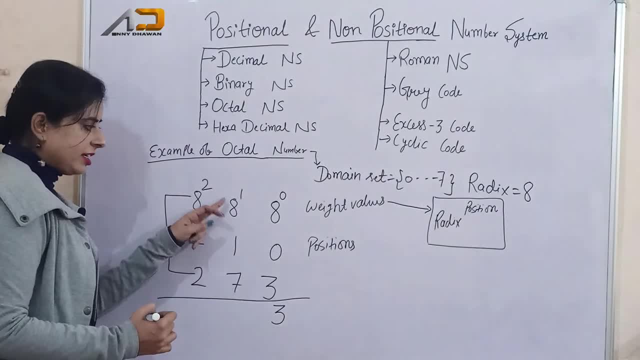 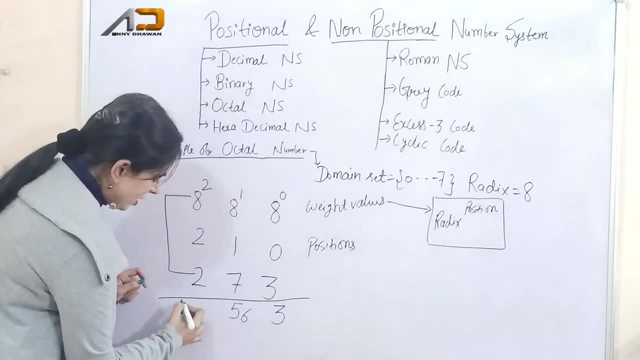 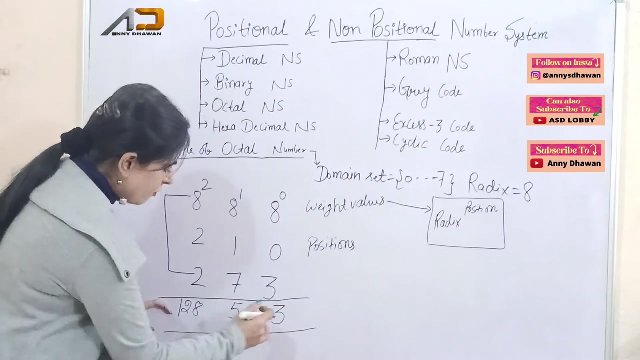 get 3 hertz. 7 multiplied by 8 raised to the power 1, you will get 56 hertz. 2 multiplied by 8 raised to the power 2, you will get 128 hertz. And to get the final answer, add the values of all the positions and you will get 187.